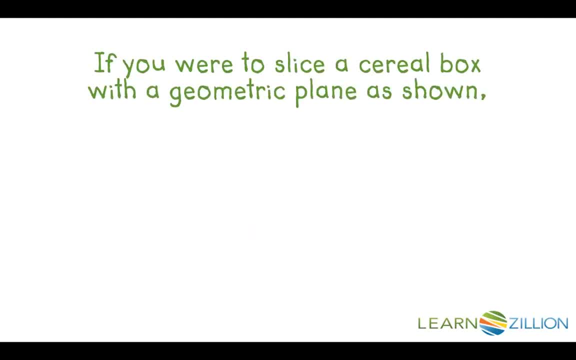 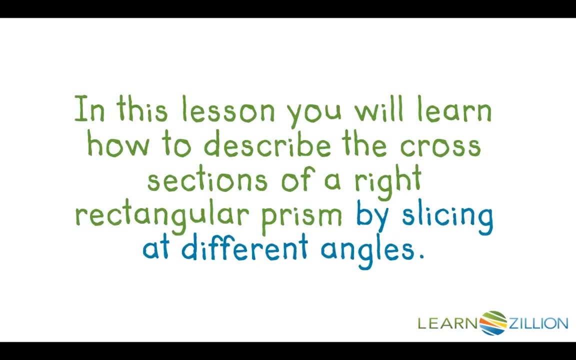 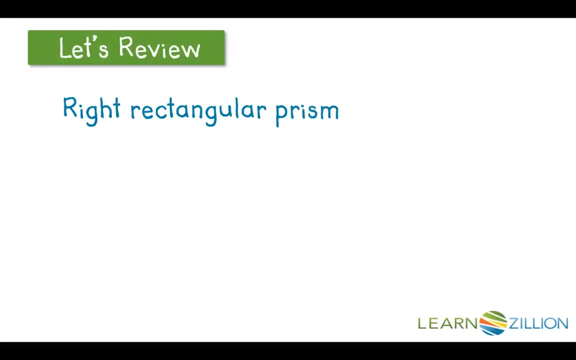 If you were to slice a cereal box with a geometric plane as shown, what shape would result? In this lesson, you will learn how to describe the cross-sections of a right rectangular prism by slicing at different angles. Let's review. In this lesson we will use a geometric figure called a right rectangular prism. 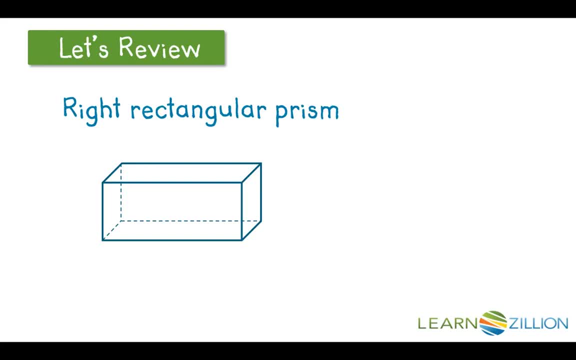 It looks like a box. It's made up of six faces that are shaped like rectangles and they meet at right angles or 90 degree angles. We will also use a plane. Imagine a sheet of paper that is infinitely tall and infinitely wide, but very, very thin, and this could represent a plane. 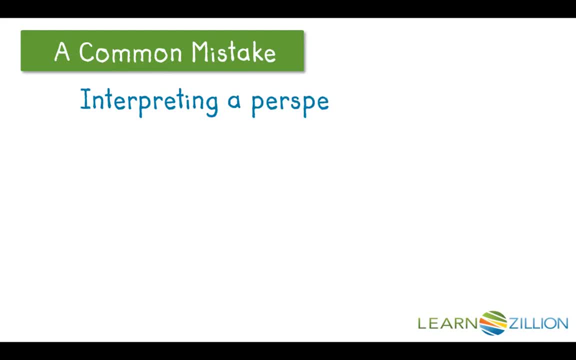 A common mistake: Interpreting a perspective differently. You may be drawing as though you were looking at it straight on. For example, here is the right rectangular prism. again, Focus on the top face. From this perspective, it looks like a parallelogram, doesn't it? 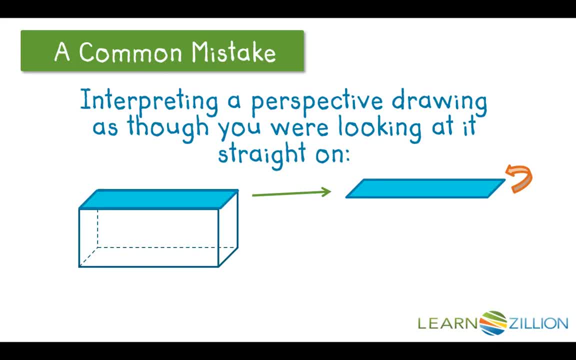 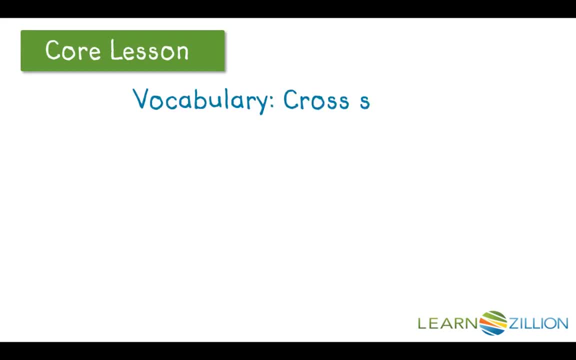 But if we stand it up and look at it straight on, we will see that that top face is actually a rectangle. Some important vocabulary that you will need to know is the word cross-section. A cross-section is the two-dimensional shape that results from cutting a three-dimensional shape with a plane. 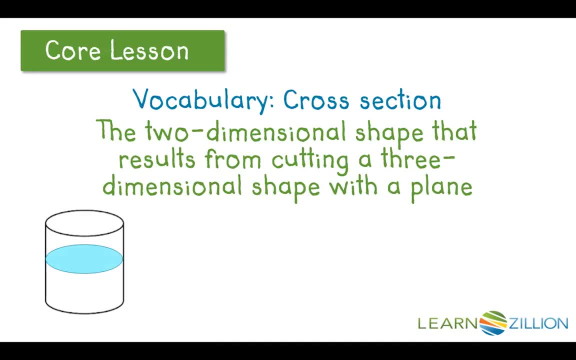 A familiar example might be a circular glass of water When it's sitting on the table. from this perspective, it appears that the water surface is an oval, But in fact, if we stand up and look at it straight on, we will see that that cross-section is actually a circle. 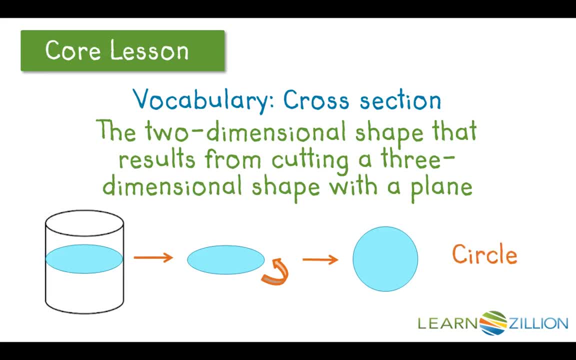 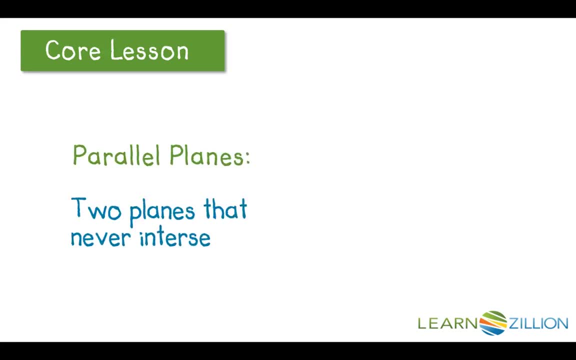 The surface of the water is called the cross-section. Two planes are parallel if they never intersect. We will be using parallel planes in this lesson. Imagine the floor of a room and the ceiling of the same room. These might represent parallel planes. We will also use perpendicular planes. 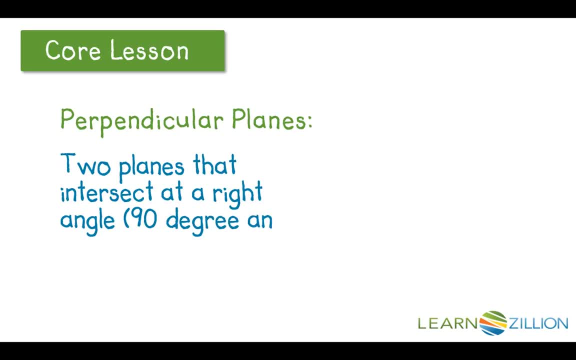 This means two planes that intersect at a right angle, or 90 degree angle. Again, think about the floor of a room, but this time imagine one wall of that room. Because they meet at a right angle, the wall and the floor would represent perpendicular planes.